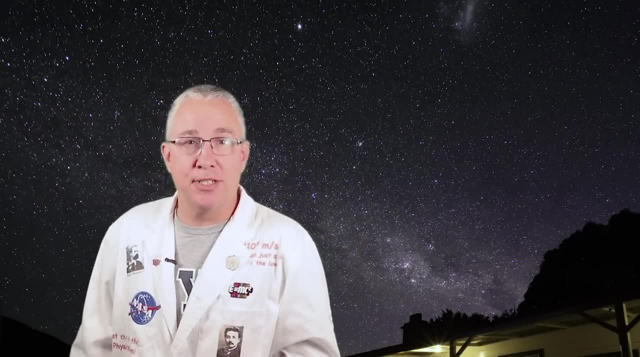 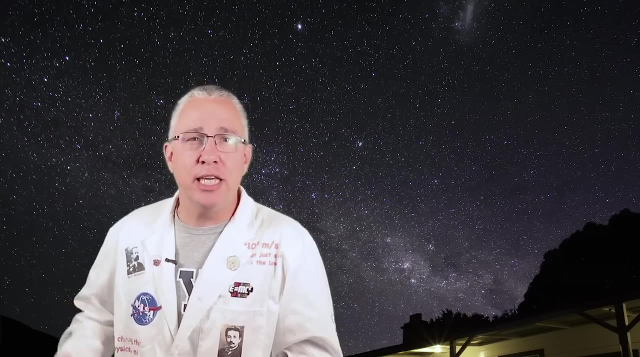 When you look up at the sky at night, you will see thousands of stars. For all intents, they look like pinpricks of light. They may have slightly different colours, but in essence, about the only thing you might notice is that some are brighter than others. 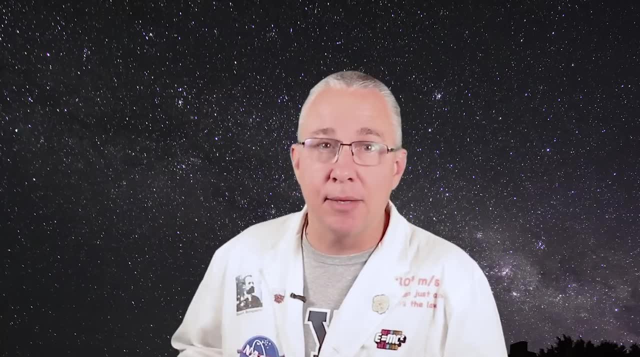 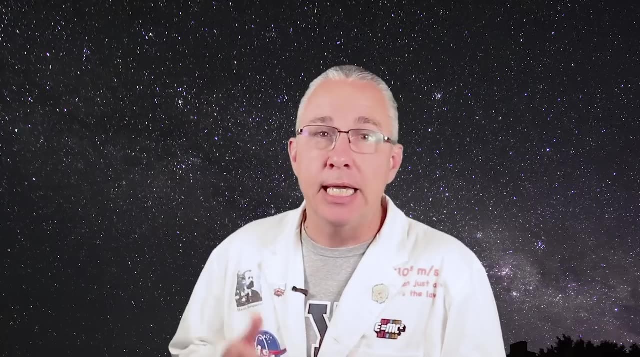 But we can learn so much more about stars if we analyse the light that comes from them, And in this video I'm going to discuss how astronomers use spectroscopy to determine four properties of stars: Its composition, its temperature, density and relative motion. 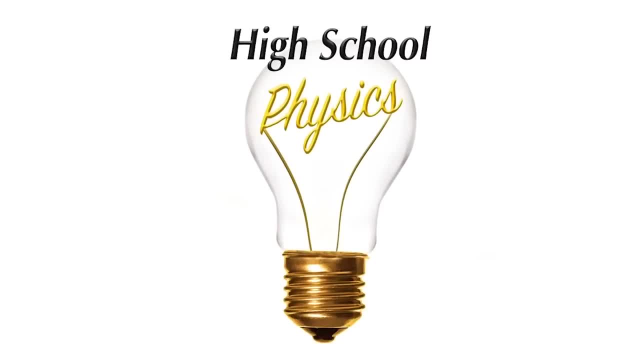 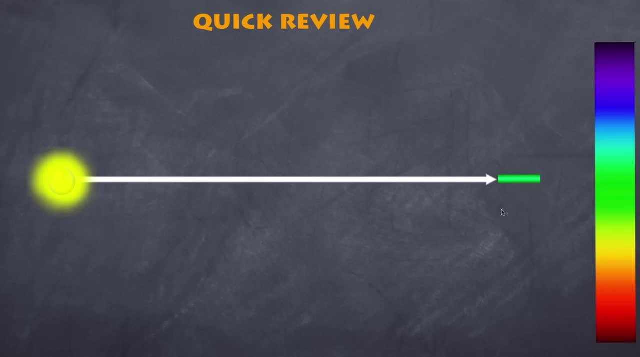 So stay tuned. Now, before we start, let's have a quick review of spectroscopy. I do have a video on the introduction of spectroscopy. If you look at the link above and also at the link at the end of the video, you'll know that light, of course, is made up of many wavelengths, many frequencies. 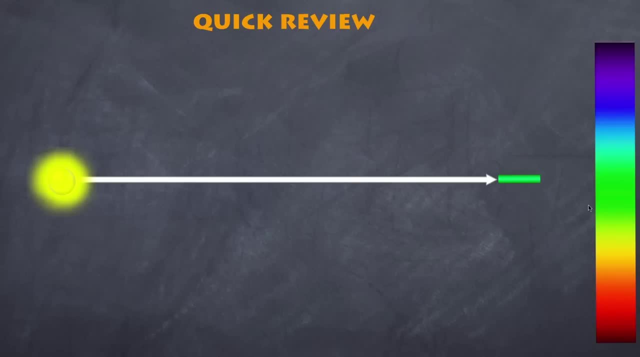 And if we spread out their wavelengths or spread out their spectra, we get this continuous spectrum from long wavelengths to short wavelengths. If we pass that light through a gas, then certain frequencies or certain wavelengths of light are absorbed by the gas and we'll get the 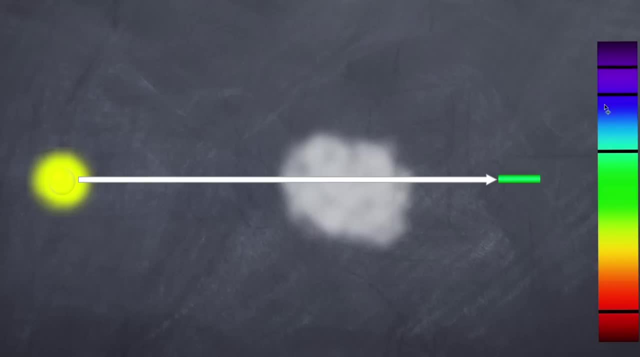 continuous spectrum minus these wavelengths, And so what we have here is an absorption spectrum, And in this case, these are the lines that represent what hydrogen would remove from the spectrum. If we were to allow the gas to heat up, it may emit that light. It'll be. 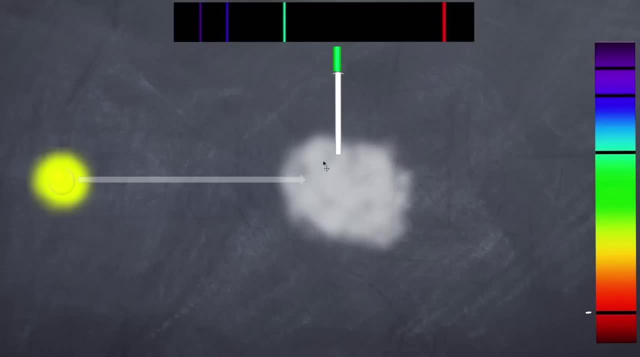 only specific due to the chemical nature of this gas. So in this case we have emission spectrum, And so these are the lines that represent again hydrogen, And you'll notice these two are complementary. So the lines that are missing here are the lines that are up here. Now let's start. 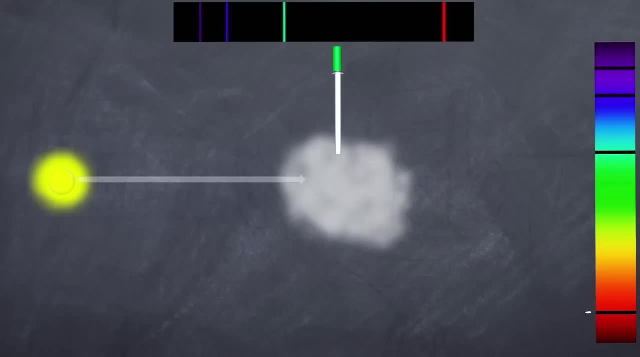 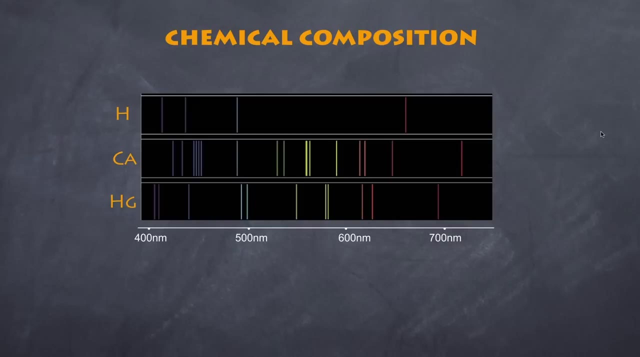 looking at how spectroscopy is used in astronomy. So the first thing is chemical composition. And before we look at the chemical composition of, let's say, our sun, let's remind ourselves that we have here three emission spectra for three different elements. So here we have hydrogen. 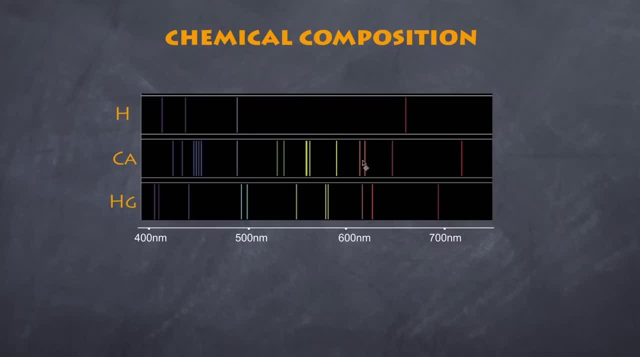 here we have calcium and here we have mercury, And you will see that the pattern of lines are very different. In fact, they are sort of like the fingerprint for each of these elements, because each of these elements remove very specific frequencies- if it's an absorption spectrum. 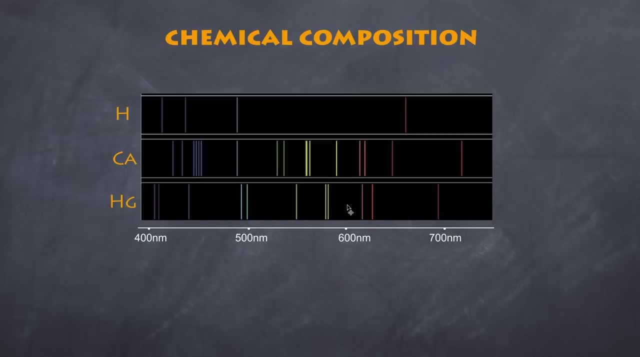 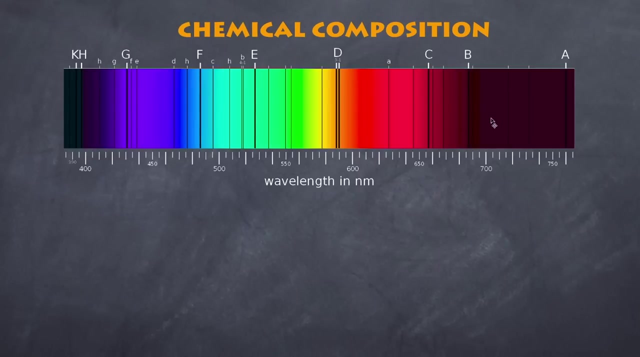 or emit very specific frequencies if it's an emission spectrum. So in other words, if you know the pattern here, if you know the wavelengths that are associated with the emission spectrum, you can determine the element that's causing that. So now let's have a look at the spectrum of our sun And you'll see we have a whole series of 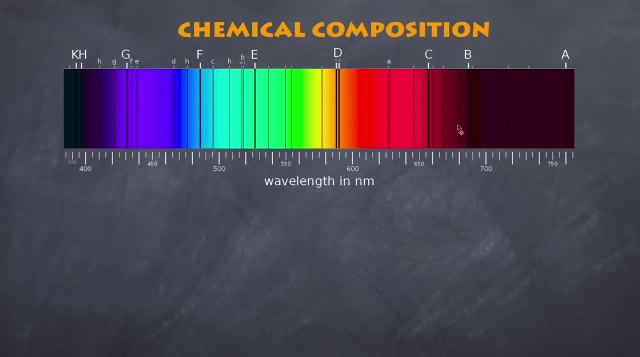 lines, And this, of course, is an absorption spectrum. Now, all of this is due to the light that is passing through the photosphere of the sun. Now, that is a gas layer around the sun that is a little cooler than the surface of the sun, which means that gas is going to remove, or 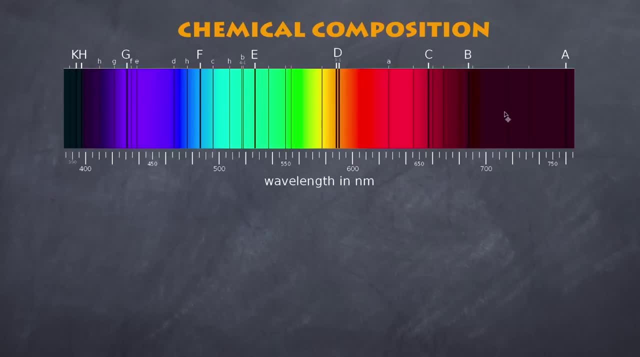 absorb some particular wavelengths depending on the chemical composition of the photosphere. Now, this is a very important element. So if you have a set of lines, often referred to as the Fraunhofer lines, they don't represent a single particular chemical. There's a whole series of chemicals. 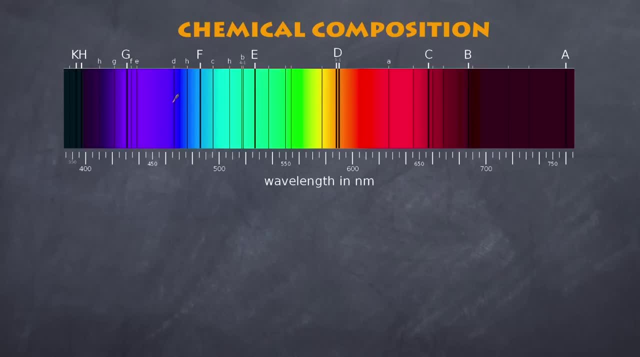 that are causing this, But if you know the positions, you can determine which chemicals they are. So, for example, if we look at G over here, we look at F over here and C over here, these are all lines that are associated with hydrogen. 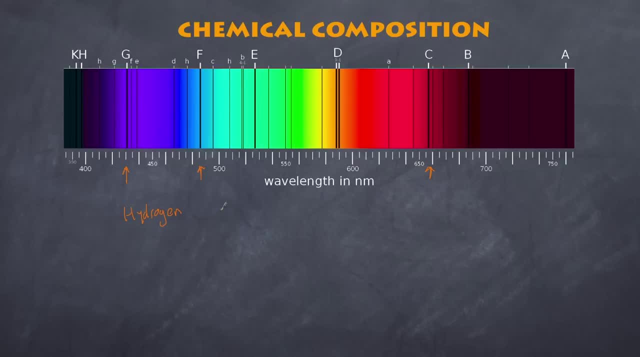 And that's not surprising. The sun, a star, ultimately- is mainly hydrogen. If we look at these sets of lines here, that's indicative of helium, And again, that's not surprising because hydrogen is being fused into helium. That's the process of which the sun works. 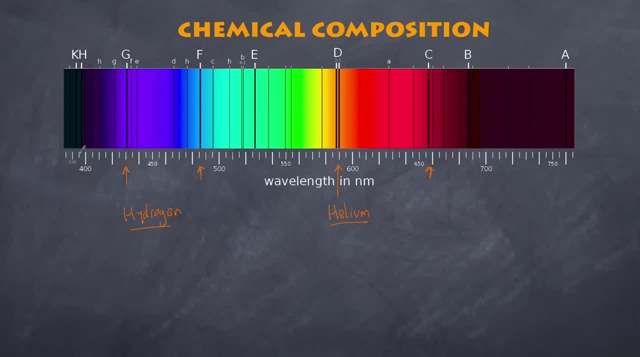 But there are a whole series of other elements here. I'm not going to go into great details but for example, K and H over here are indicative of the presence of calcium ions. So if you know wavelengths are absorbed by various chemicals, you can determine the chemical composition. 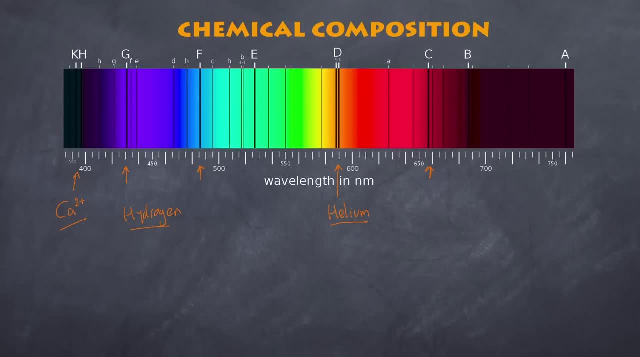 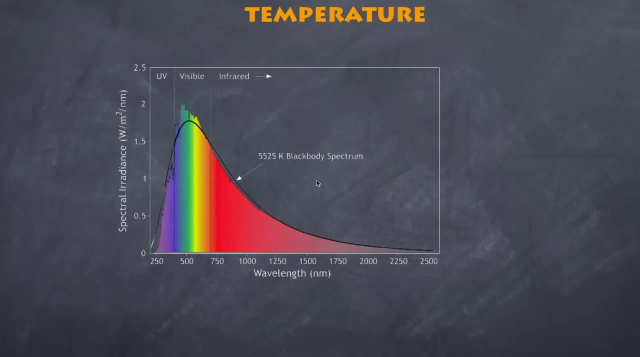 of a star by simply analyzing its absorption spectrum. Now, before we look at temperature from a spectroscopy perspective, we need to quickly look at what we refer to as a blackbody curve, And what really this is representing is all the wavelengths that is coming off a star. 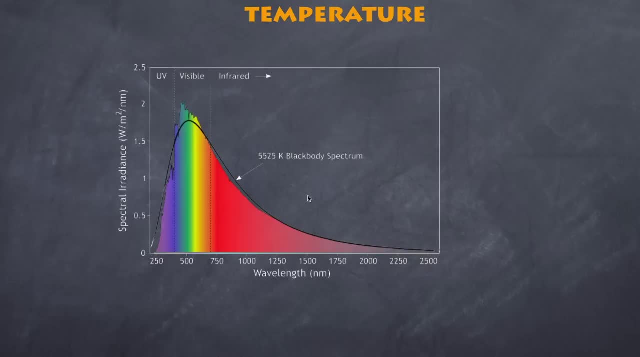 which, in essence, is what we refer to as a black body. Now you'll see that a star does not give off a black body, It's just a black wave that comes off it. So in this example, you'll see that the maximum wavelength we get is in the roughly green, yellow range of the spectrum. 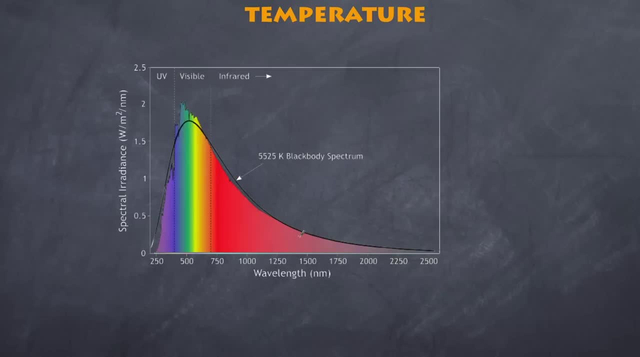 Down here you'll see we have. yes, surely red is giving off, but it's less intense. And then in this section over here, this is all infrared. So obviously there is lots of infrared coming off, but it is significantly less in proportion to the light that's coming off. 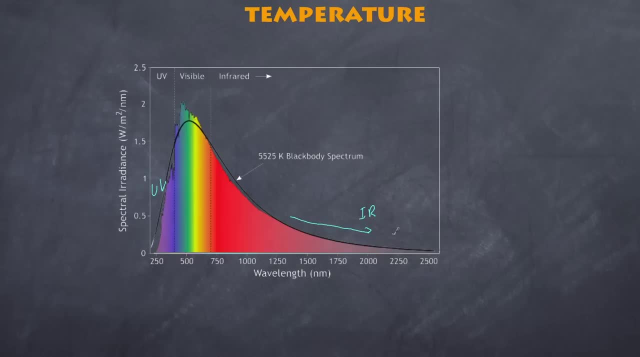 Yes, there's also ultraviolet coming off, but it significantly drops off. If we keep going this way, we would also get microwaves and radio waves as well. So that gives you an instance that all the wavelengths are given off, but at varying. 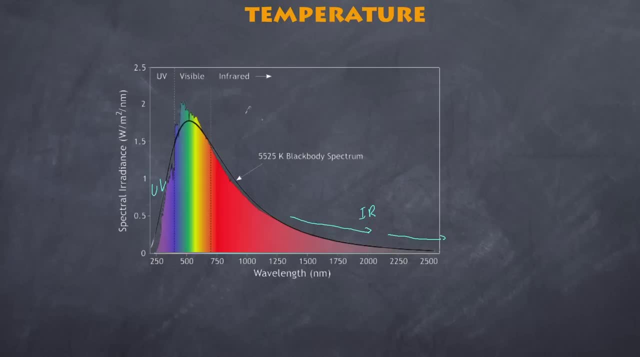 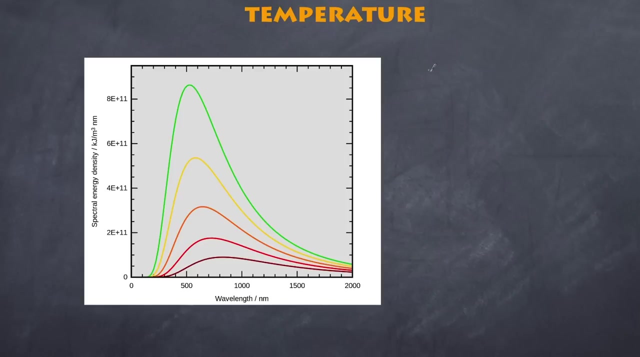 intensities. Now, what is special? Now, if you look at the wavelength that has the greatest intensity, we can determine the temperature of the body. So that gives us Wien's law. So Wien's law in essence says this: is that the temperature 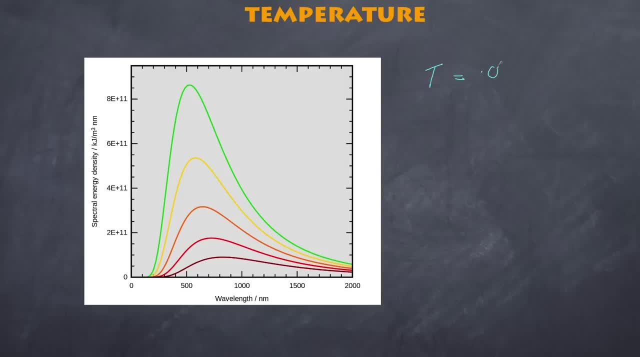 is equal to a constant which is 0.00289 divided by the wavelength that is of the greatest intensity. So, for example, a star that has a black body curve looking like this, its wavelength is in this range over here and has a temperature of 3,500 Kelvin, You'll see. the next one is a. 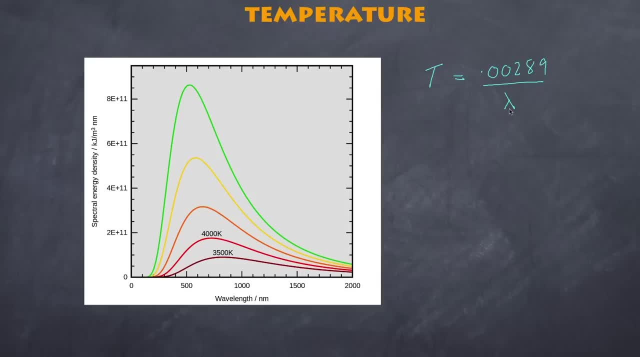 higher temperature and you'll see that the wavelength gets smaller, which is consistent with Wien's law, which is an inverse relationship: The hotter it gets, the further the peak moves towards the left, That is, the temperature increases as the wavelength decreases. If we then analyze all stars that we can see and use the black body radiation curves, 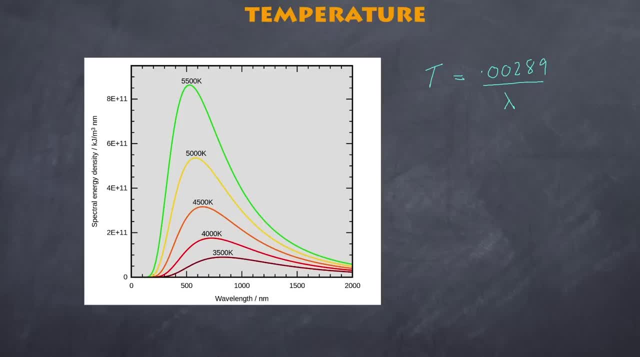 we can then classify stars according to various spectral classes, And these spectral classes were developed in the early part of the 20th century and they have classes that have letters O, B, A, F, G, K and M. Now you can see that O-class stars. 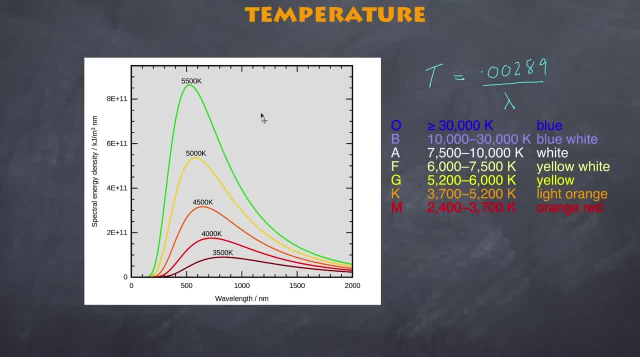 are generally considered blue, That is, there's more wavelengths in the blue, So we look at them from a blue perspective. So therefore, their temperature is greater than 30,000 Kelvin And if we go down the scale, we eventually get really cool stars, relatively speaking. 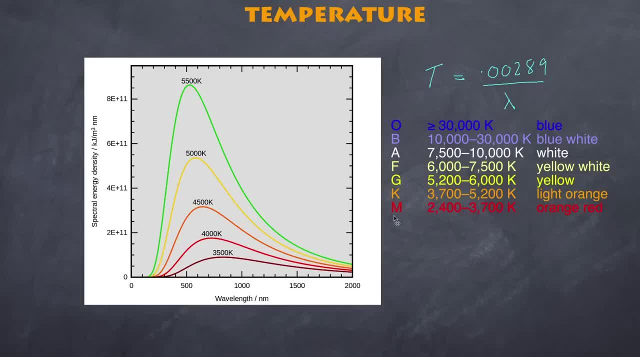 of around 2,500 to 3,500 Kelvin, And that's the M-class star. So that's this curve here. Now, why is that useful? Well, we then want to look at this classification. We can then start looking also at the spectra. 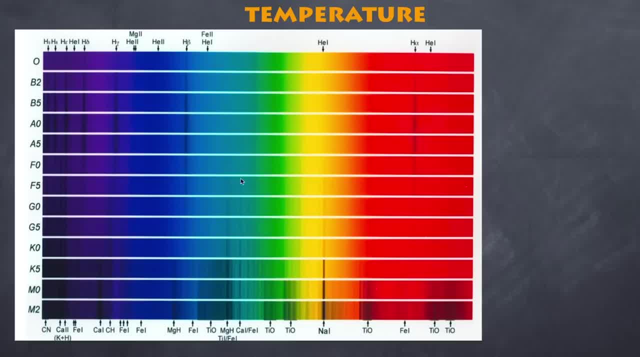 of these stars. So now here we have, a chart that shows you the absorption spectra for various classes of stars. Now the numbers here represent subclasses or subgroupings of each of those classes. So for example, A-class, which is over a particular temperature, can be divided anywhere. 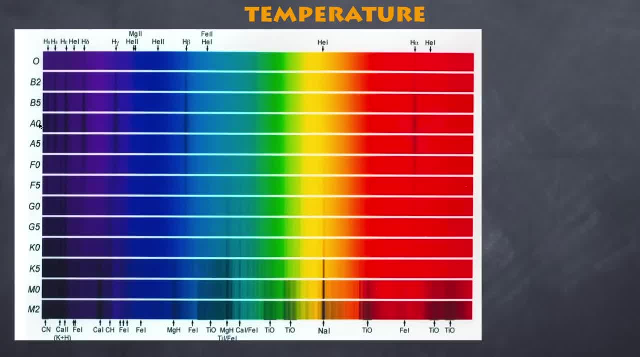 between A0 and A9. And so, therefore, the absorption spectra can be divided anywhere between A0 and A9. And so, therefore, the absorption spectra can be divided anywhere between A0 and A9. And so here we have two A-class stars, but the A5 is a slightly cooler than, let's say, A0.. 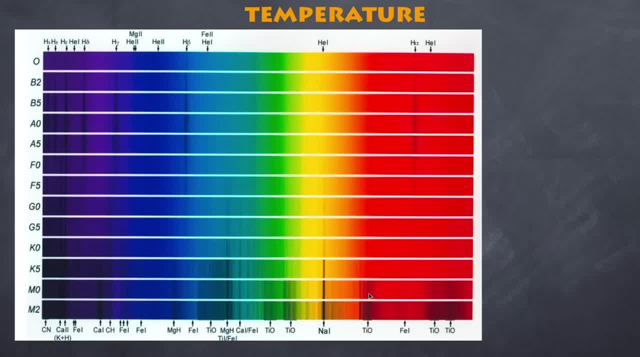 What you'll notice here is that the absorption lines are not all the same. So if we analyze the absorption lines of a star, we can determine more in detail the temperature of that star, because certain temperatures have certain features in terms of their absorption lines. The first thing: 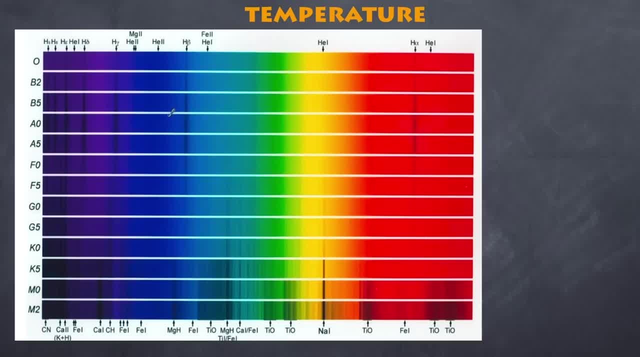 we'll notice is that if you want to look at the A-class star, you'll see that our hydrogen lines here and here and here are significantly strong, And so that's one of the hallmarks of an A-class star: They have very strong hydrogen lines, but weaker in other lines. If we look at O and F, 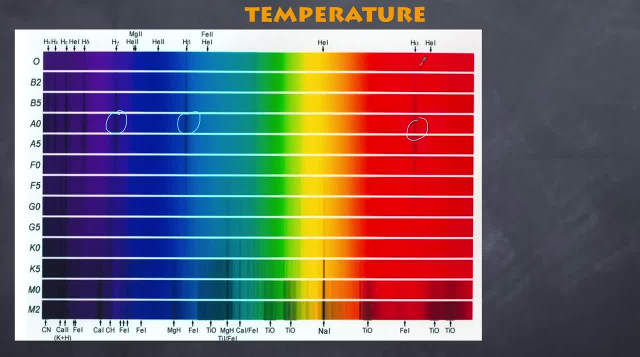 there. we'll notice that the hydrogen lines are there, but they're somewhat weaker. But how do we differentiate between our O-stars and our F-stars if they're weaker ones? Well, we now have calcium lines here which are now stronger. So one of the hallmarks of, let's say, an F-class star is: we have 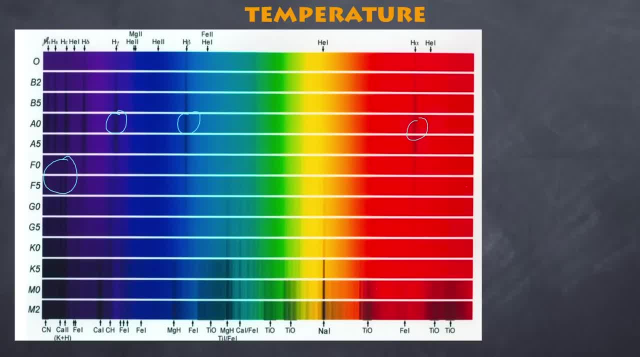 weak hydrogen lines, but we have stronger calcium lines. So you'll notice that the calcium lines in the O-class star is significantly weaker. If we then go to G-class stars, you'll see that the hydrogen lines are weaker again, but now you'll also start to get obviously stronger, And so 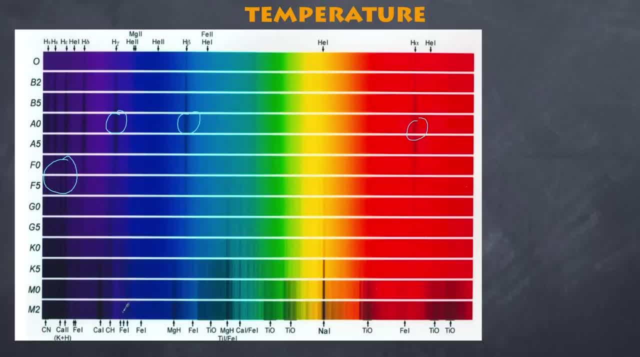 you'll notice that there are some strong calcium lines, but also some other metals appearing as well, And you can see these fine lines here, And that is because the temperature is lower, and so we'll find that the energy for the elements required to absorb and re-emit light is of the 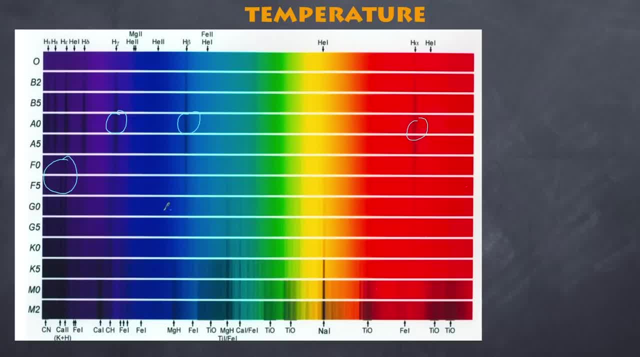 right level for it to occur. So you'll see that certain elements are visible here which aren't visible at all up here. Then calcium becomes significantly stronger. So one of the hallmarks of a K-class star is that the calcium lines are at their strongest. And then we get to M-class stars Here. 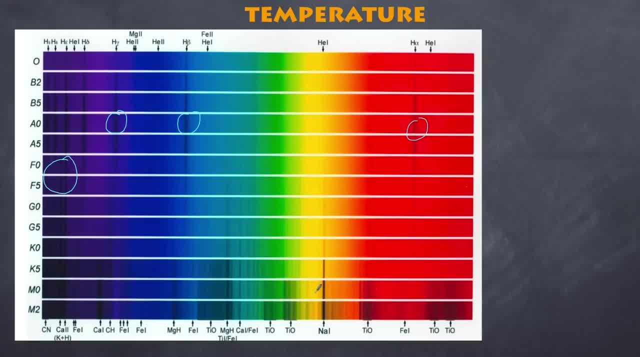 the temperature is so low that even molecules can exist and absorb and re-emit. And so you'll notice here that not only do we have lines of elements, but then we also have lines of titanium oxide, for example. So in that case, these cool stars you can see, have very 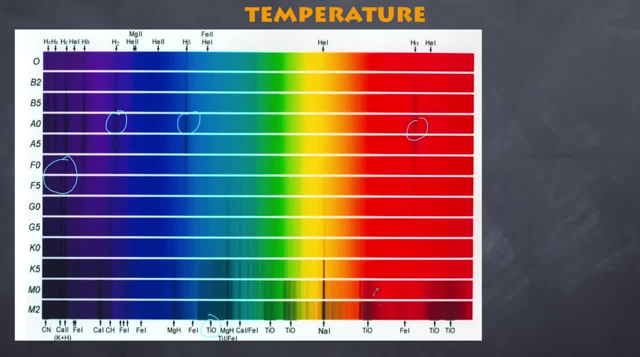 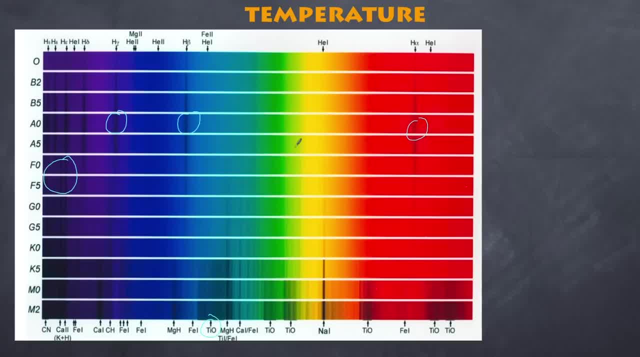 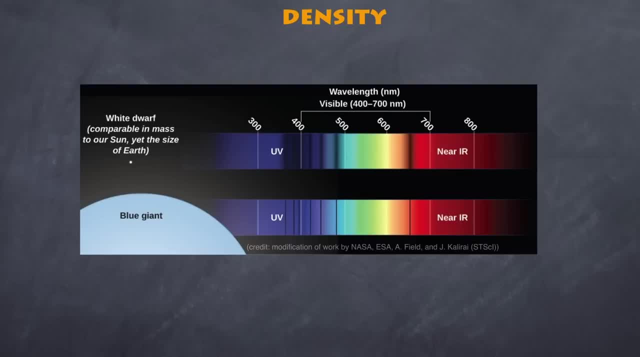 spectral lines allows us to determine the temperature simply by looking at the strengths of the various lines. Now, the density of the photosphere has an impact on the quality of the lines as well, If there is a great density in the photosphere, and so therefore the pressure. 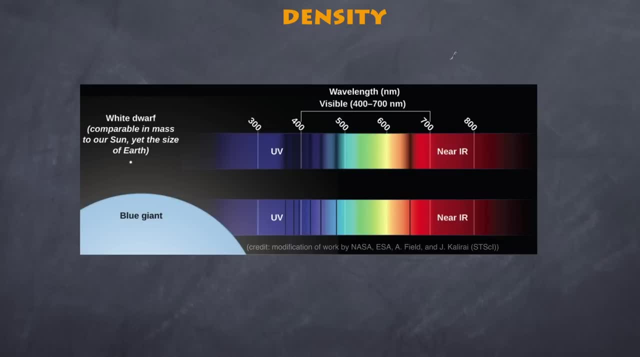 is high, then what you're going to discover is that there's going to be lots of collisions in that photosphere, And because of the lots of collisions you're going to find you're not going to get really smooth, clear lines. And so here we have. 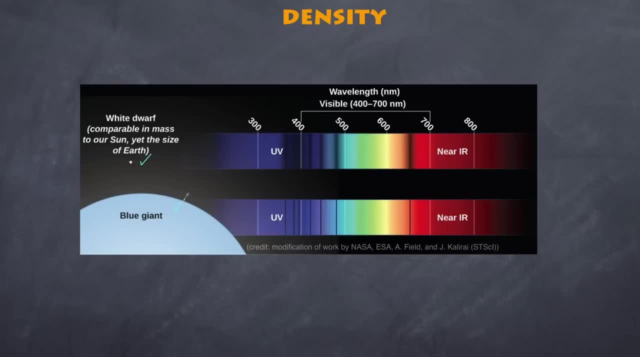 a white dwarf and here we have a blue giant And they both have, relatively speaking, similar temperatures And these are particularly high temperature stars. But because of the nature, because of their density, blue giants are fairly spread out, so therefore they have low density. their spectral lines differ. So you'll see, in the highly dense 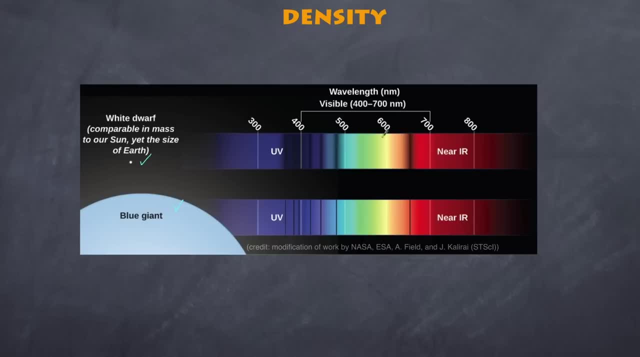 and compact white dwarf. you can see that the spectral lines, although they are aligned with the ones down below, you'll see that they're very fuzzy. Where, here with the blue giant, where the density is significantly less, there are less collisions in the photosphere? 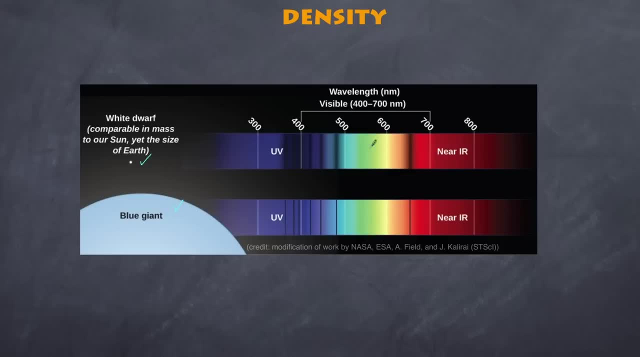 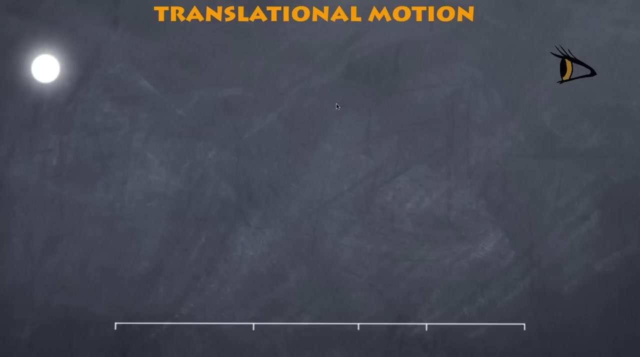 we're going to find much finer spectral lines. Examining the position of the lines tells us the composition. Examining the types of lines tells us its temperature, And the fuzziness or the thinness of lines tells us its density. Now the next thing I want to look at is 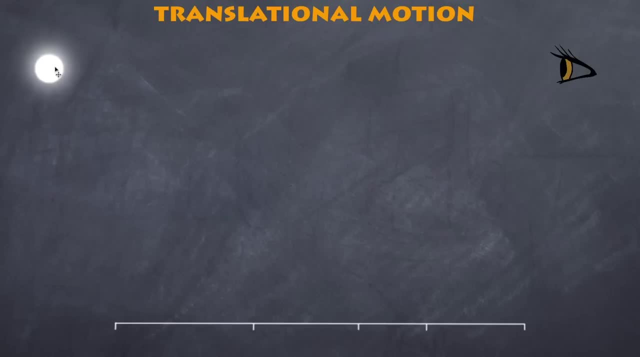 translational motion. What do I mean by that? Well, is the star moving towards you or away from you? And can we tell whether a star is moving towards you or away from you simply by analysing its spectra? And we can. The first thing is to say: well, what does a 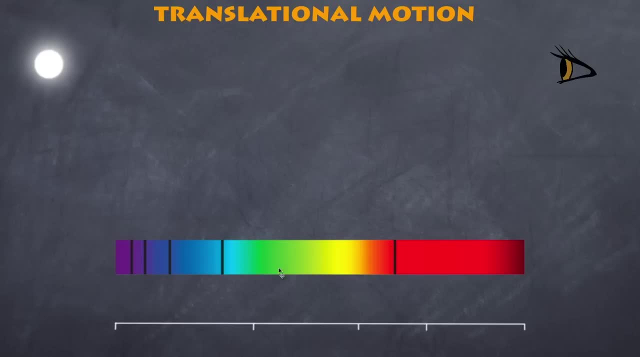 star look like. if it's stationary, So you will get a normal spectra, So you'll have a wavelength of light- and I'm just going to be representative- that looks something like this. So you're going to have sort of the wave coming a little bit more close with its characteristic wavelengths, or 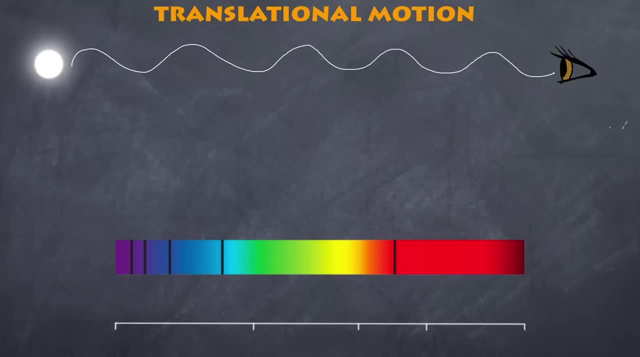 range of wavelengths. I'm just using this as a diagram here, But what happens if the star is moving towards you? Well, if the star's moving towards you, we're going to find that the wavelength is a little bit smaller. So in other words, it sort of 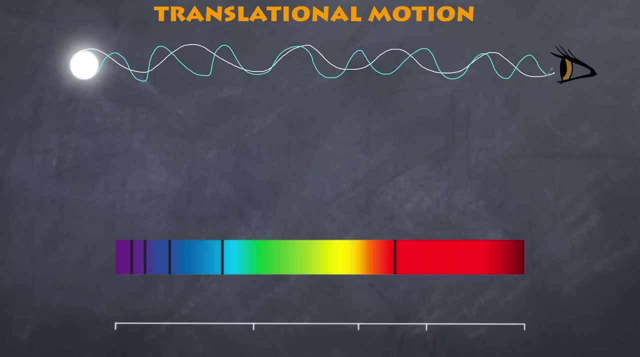 pushes closer together, like so, And we call this a Doppler shift. Now, it isn't a Doppler shift where the speed of the wave changes, but the frequency does increase or the wavelength decreases, And what that does to our spectra is that it shifts it towards the blue. You'll see that each of these 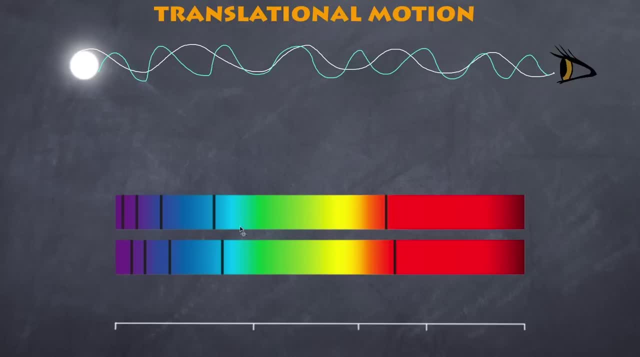 lines is moving at a higher speed. so you can see that the blue range is moving and each of the lines line up sort of as in with relative to each other, but there is a shift towards the blue, that is, each of the lines have moved just a little bit in that direction and so we say it's blue shifted. 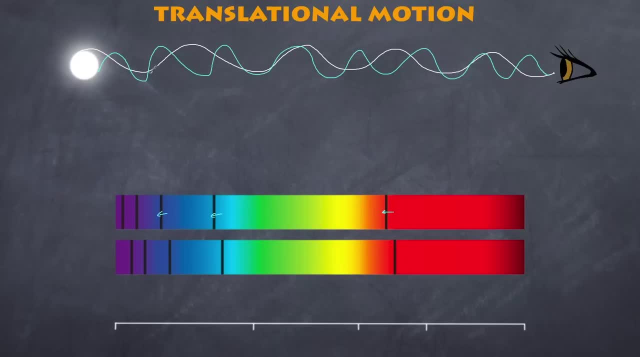 the amount of blue shift determines, for example, how fast the star is moving towards you. now what if the case the star is moving away from you? i guess you can work out what's going to go on then. what we're going to get- and again i exaggerate this here- is we're going to get a wavelength that 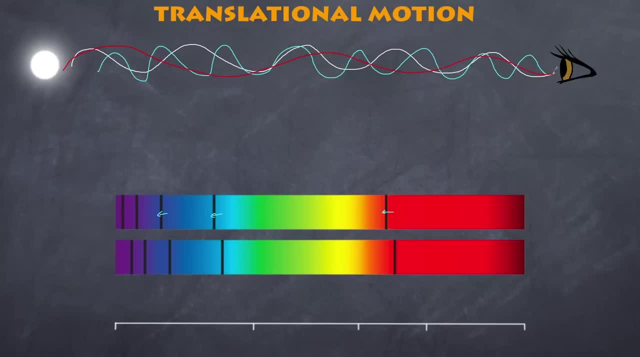 is longer. again, i'm really exaggerating this here. the wavelength gets longer, the frequency gets lower and if the star is moving away as a result, you're going to find that in this case the light causes the spectra to shift towards the red end. so we say it's red, shifted in that direction. 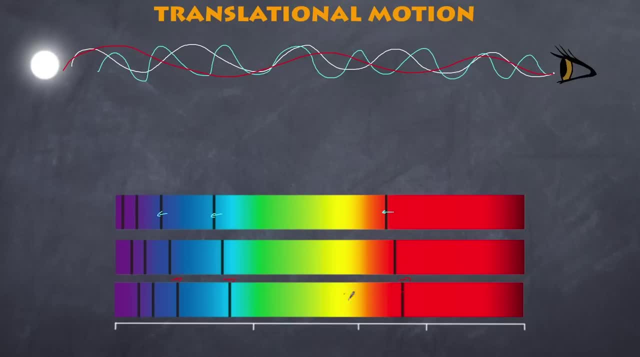 you can see, every single one of them is shifted towards the red, and again, the amount of shifting will allow you to calculate the relative motion. now, of course, it could be our motion as well. so, in other words, if we are moving towards the star, that is of course going to cause a shifting. 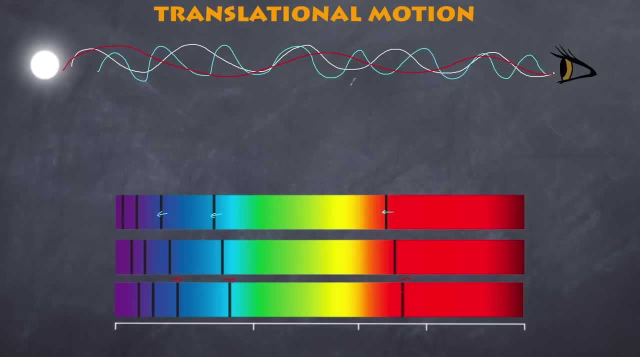 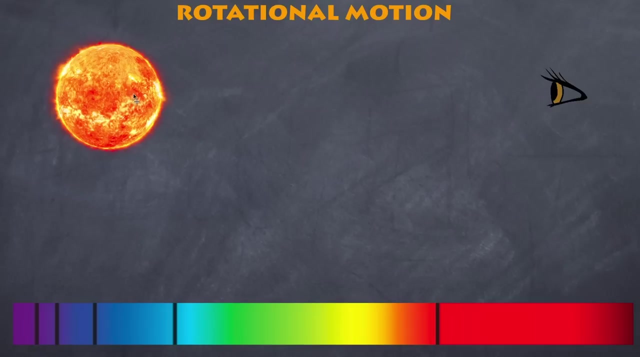 as well. in other words, that is translational motion. by looking at the shifting of the lines, we can determine the velocity, or relative velocity, between us and the star. the final one i will look at is rotational motion, and that is. a star, of course, isn't stationary. 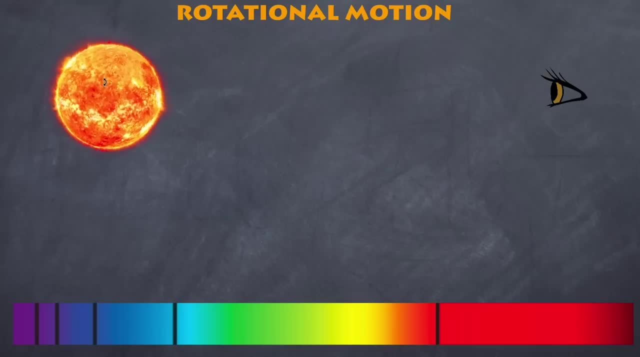 it's also going to be rotating. now, if it's going to be rotating, what does that do to the spectra? the first thing, if, is that the light at the center being moving in that direction is just going to give us a normal wavelength of light. like so, however, this far end here is moving away. 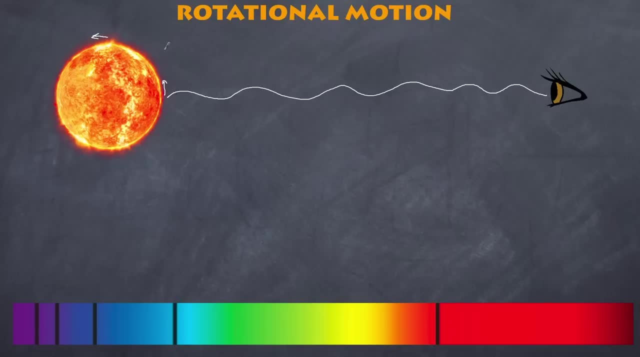 from you, so that's going to give us a little bit of a red shift. so, in other words, the wavelength is going to be a little bit longer. however, the lower margin is moving towards you, which means we're going to get a much shorter wavelength. well, not much shorter wavelength, but definitely. 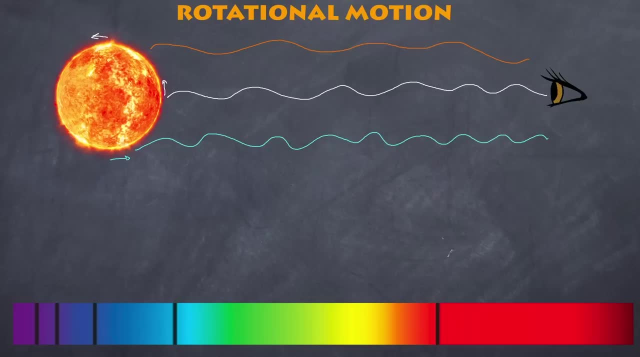 shorter, but you're going to get all three at the same time. so this line is going to not move one way or the other, but it's going to move both, and that means the lines become slightly broader. Now, this is not fuzzier, this is simply broader or fatter lines, and that's again indicative of the